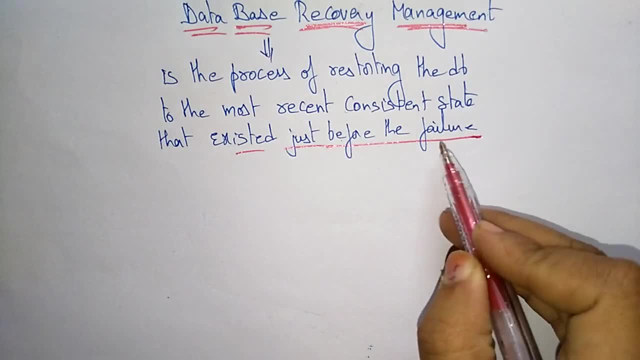 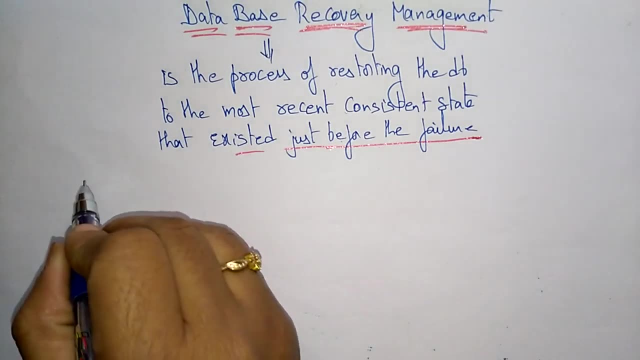 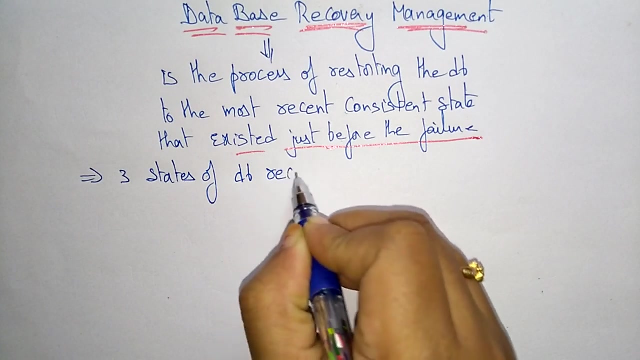 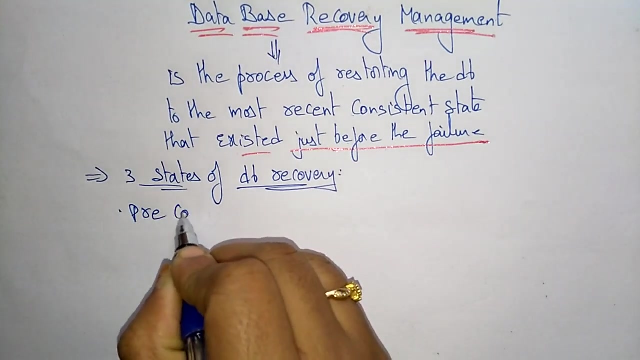 consistent state that is failed. just before the failure, that data will be restored. Okay, So let us see three states of database recovery. will be there Three states of database recovery? So those three states are: first is pre-condition, condition and post-condition. So, whatever the database you created, 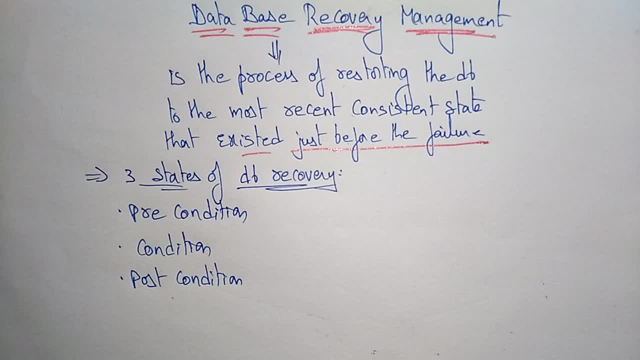 that database in any of these three states. Okay, So then you can recover your database. It may be in your computer. it may be in your computer, it may be in your computer. or it is pre-condition, or it is condition or post-condition. Pre-condition means at any. 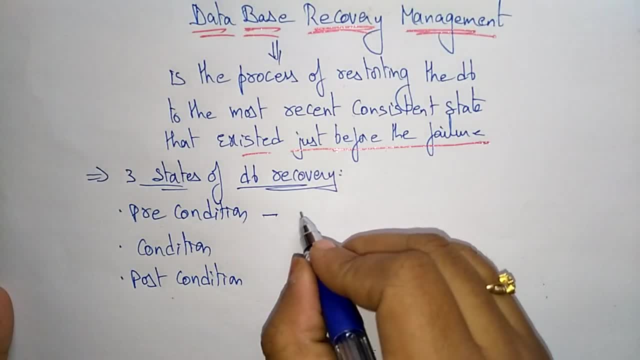 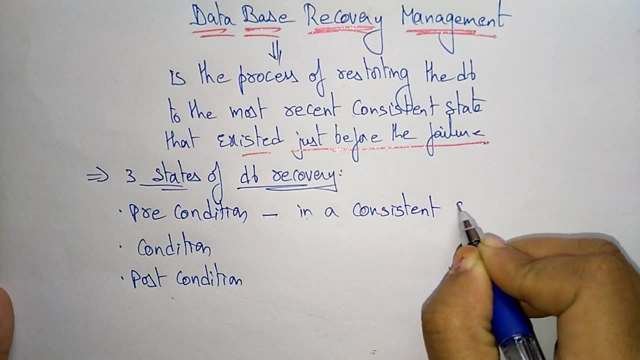 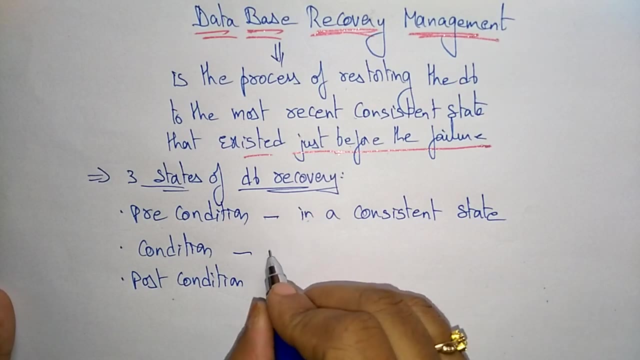 given point in the time the database in consistent state. If a database is in a consistent state before the failure, that data will be stored. So that is a pre-condition. Condition means at a particular time Means if you are doing the work at that time, so it occurs. 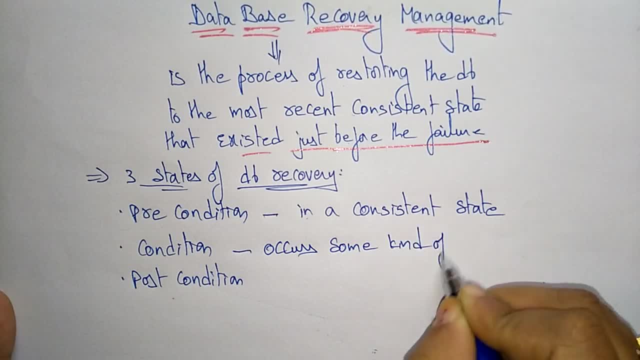 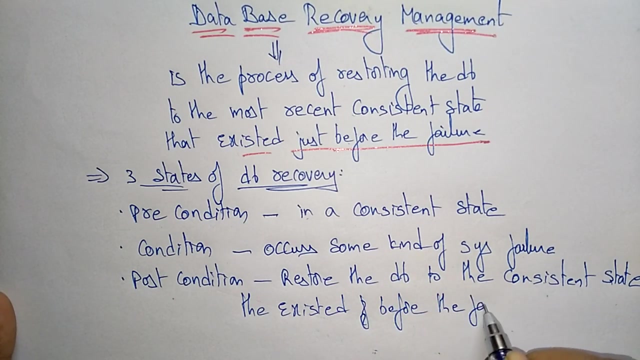 at some kind of system failure. Okay, So it occurs. at some kind of system failure, the database recovery will occur, And then post-condition means restore, Restore the database to the consistent state That existed before the failure. So these are the three states of database recovery. 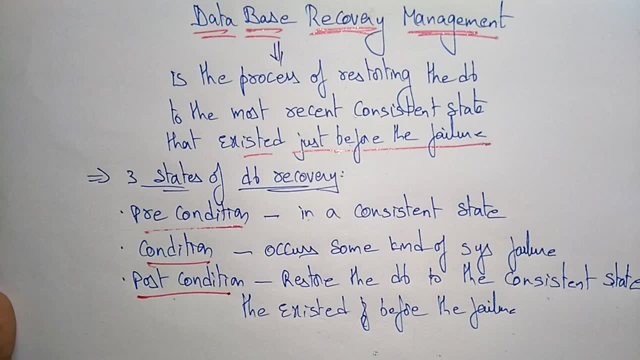 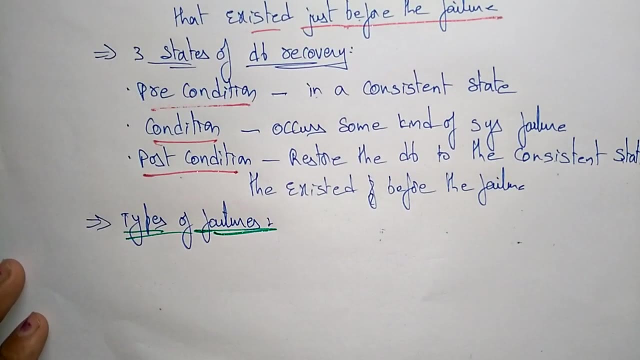 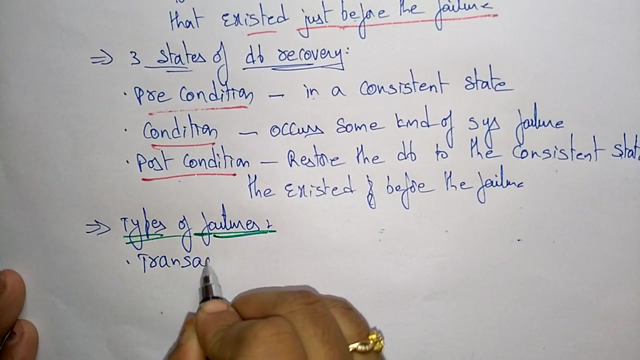 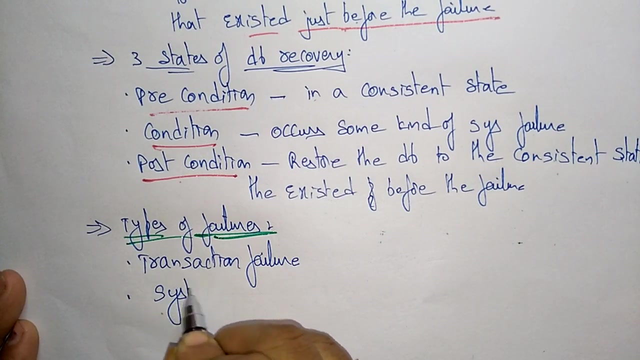 Pre-condition, condition and post-condition. Now coming to the different types of failures. So what are the different types of failures that are occurred in database? So types of failures: First one is transaction failure, Transaction failure, System failure or media failure. 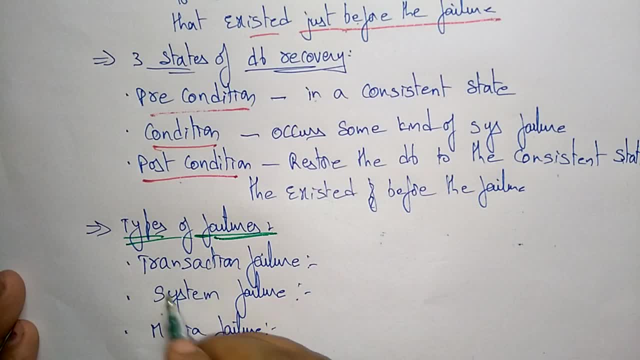 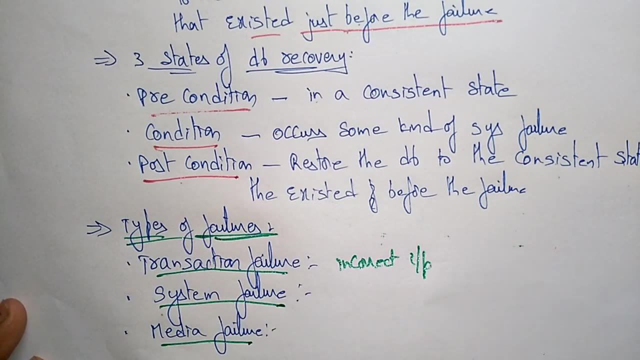 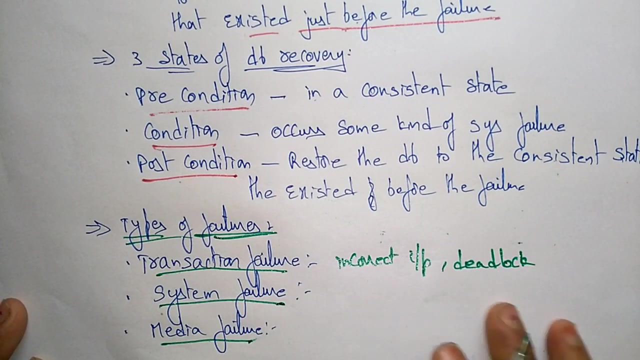 Okay, So the different types of failures are the transaction failure, system failure and media failure. system failure, media failure. so transaction failure means the transaction may fail because of incorrect input. so if you are giving any incorrect input, the transaction may fails. so if suppose deadlock is occur, so deadlock. so those are the transaction failures. what is the 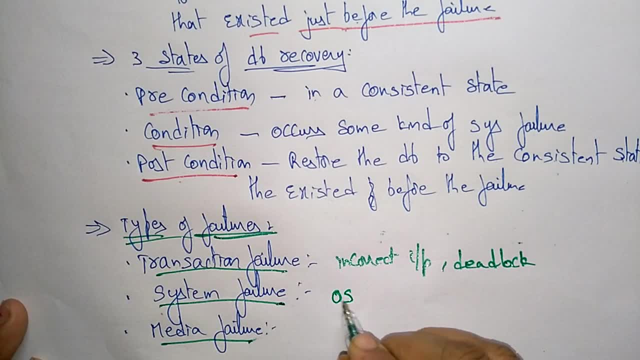 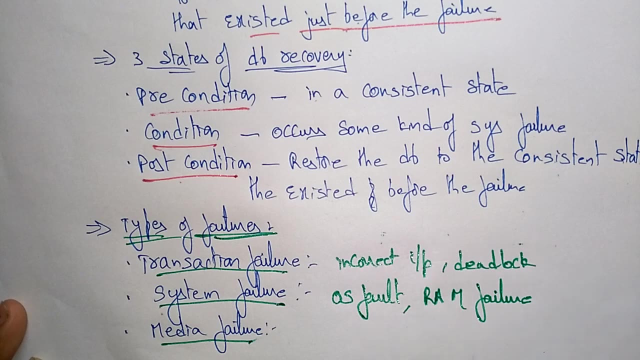 system failure. system failures is nothing but the operating system fault. if there is any fault in the operating system, the system may fails or RAM failure. suddenly the RAM gets damaged means the RAM failure like that. now coming to the media failure, media failure is nothing but the disk. 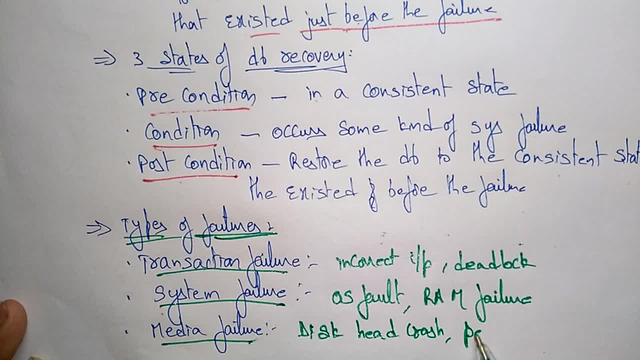 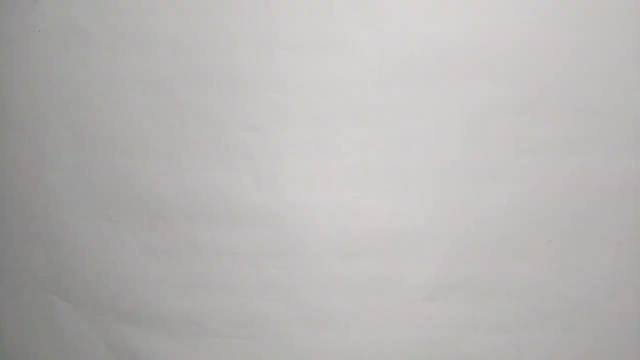 head crash power problem. okay, so these are the media failures. this is the problem. these are the three different types of failures: transaction failure, system failure and the media failure. so now come to the database basic update strategies. so these are the main basic update strategies. whenever you want to recover your database, you would you have to follow these basic 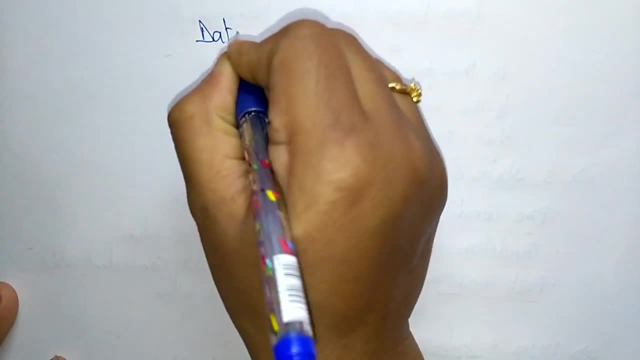 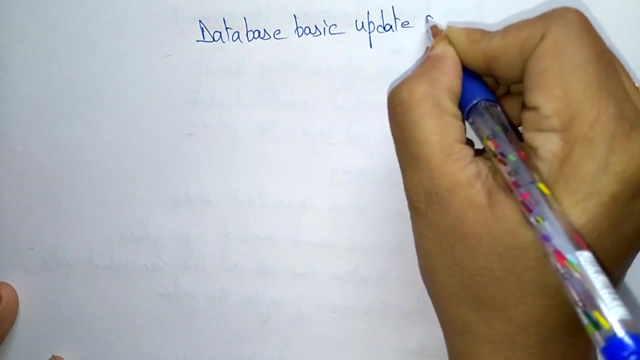 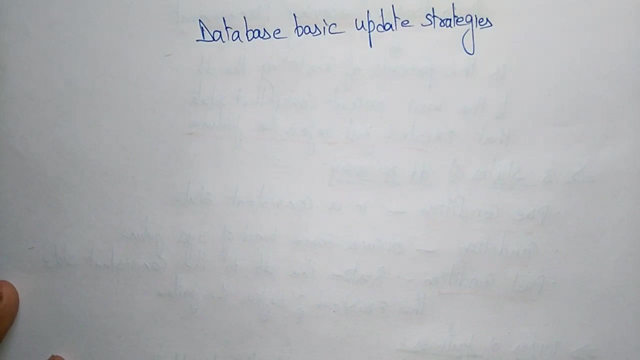 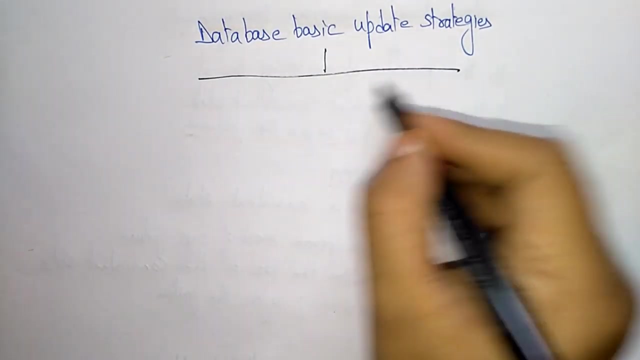 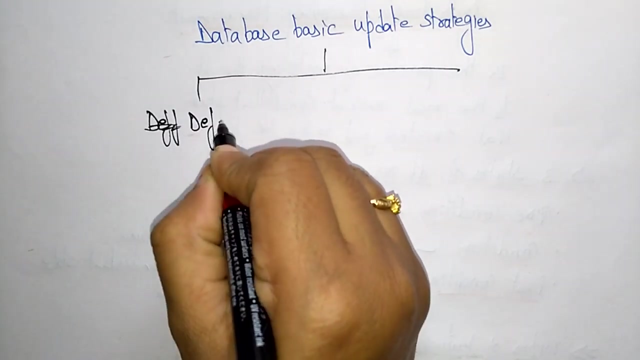 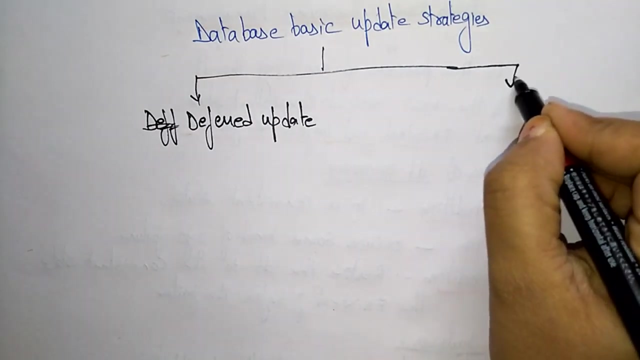 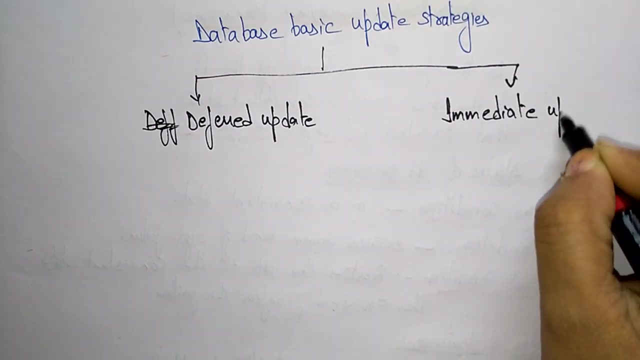 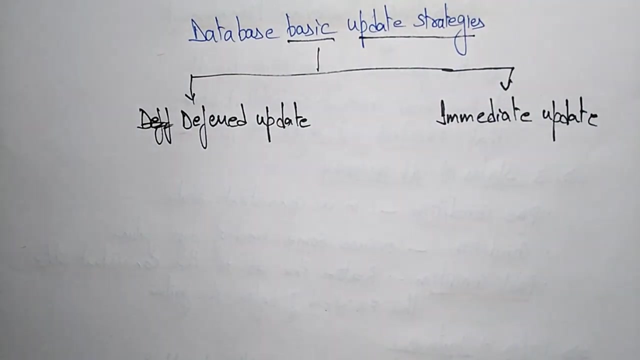 strategies database- basic update strategies. so what are these basic update strategies actually? this basic update strategies will be divided into two. one is deferred update, another is immediate update. okay, so the basic update strategies are deferred update and immediate update. so what is this deferred update and immediate update? so here, first, let us see the deferred update. 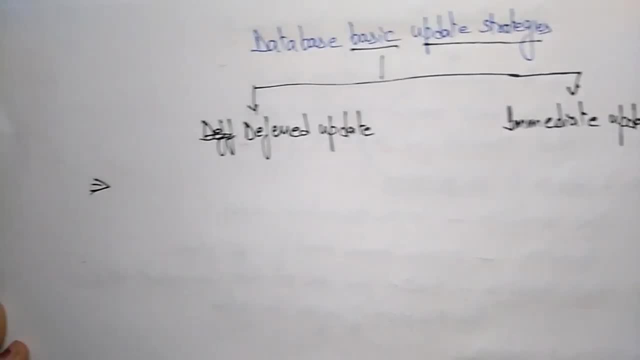 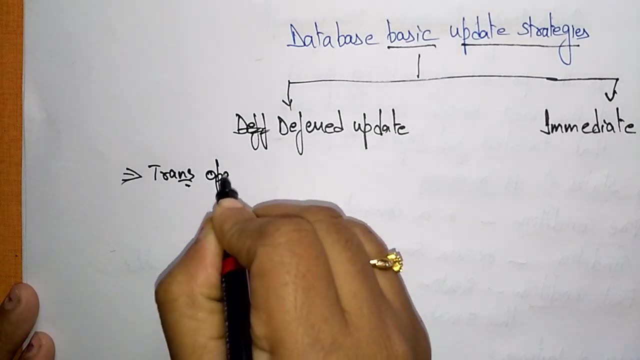 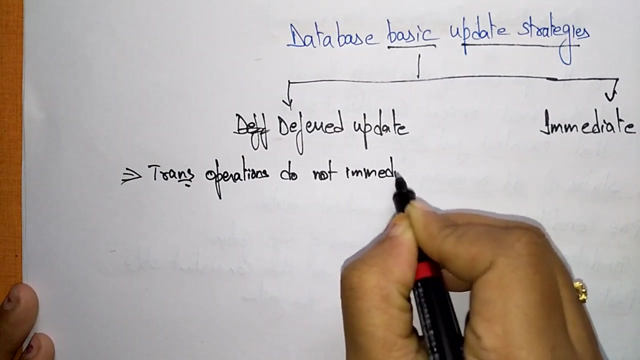 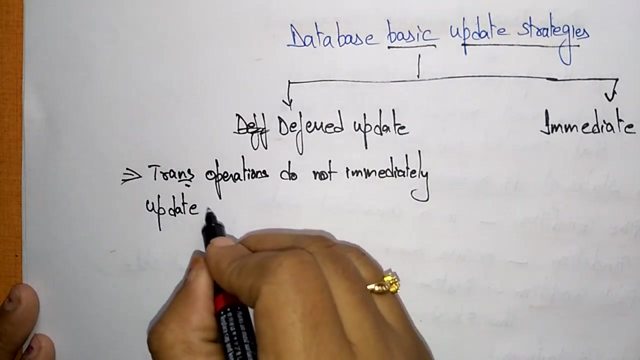 suppose your database is following the deferred update strategy. it means here the transaction operations do not immediately update, do not immediately update, update the physical database. so whatever the physical database you're using, the transactions if you are doing on that database they do not immediately update in deferred update if you use 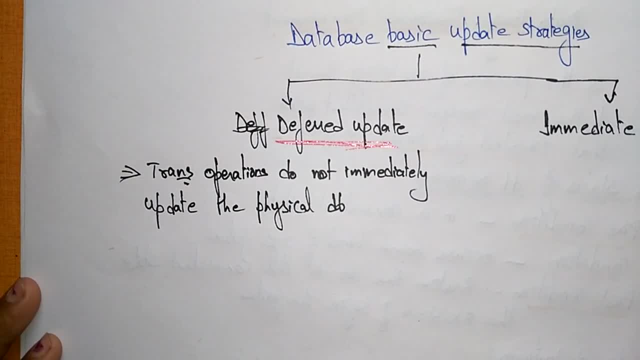 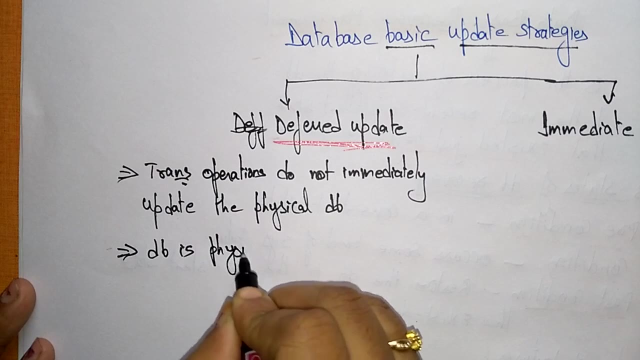 update status the transactions, whatever you are doing, those will not immediately updated. so when these transactions are updated, whenever you done the transaction with a commit statement, okay, so database is physically updated only after the transaction reaches its commit point. so whenever the transaction reaches its commit point, then only your database will be physically updated, or? 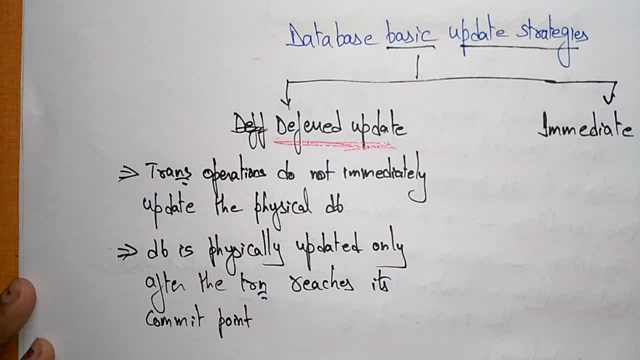 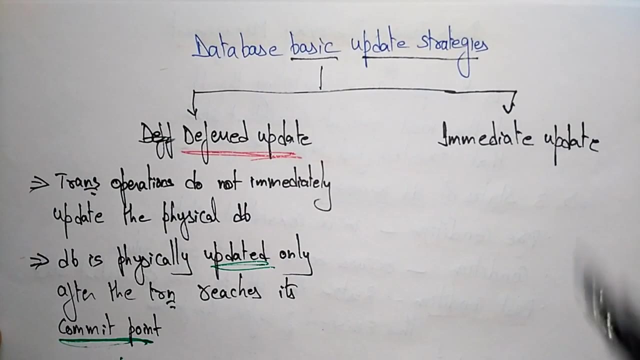 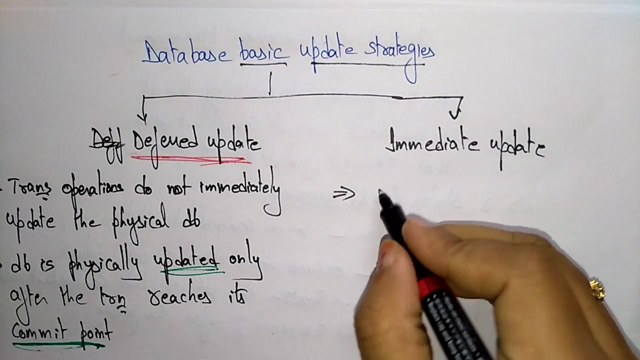 otherwise, whatever the transactions that you done before the commit point, all will be lost. okay, whenever your transactions reaches the commit point, then your database will be updated in the deferred update. so coming to the immediate. so what? what if this, if your system is in immediate update status, so what it does? so here the database is. 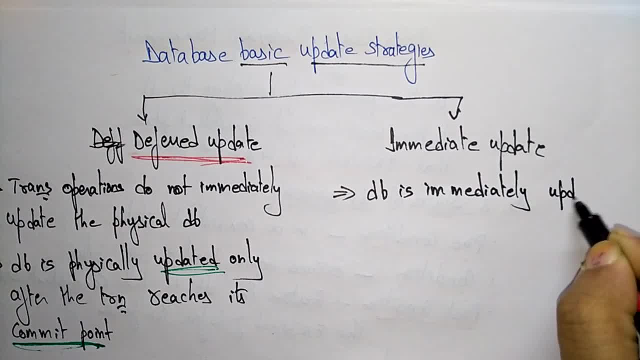 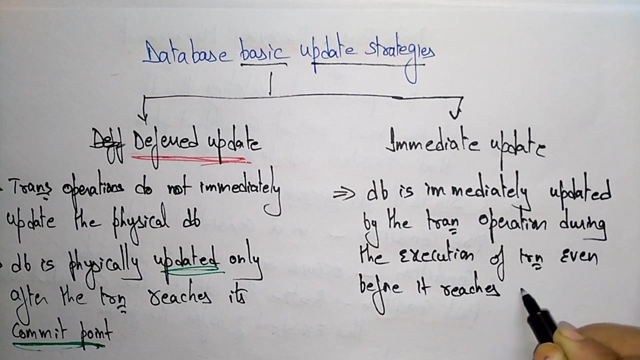 immediately updated by the transaction operation during the execution. so during at the time of execution or doing the operation, execution of transaction even before it reaches commit point. okay, so be even before it reaches the coming point. whatever the transactions you are doing, they are automatically updated. suppose, if you see in your word uh. 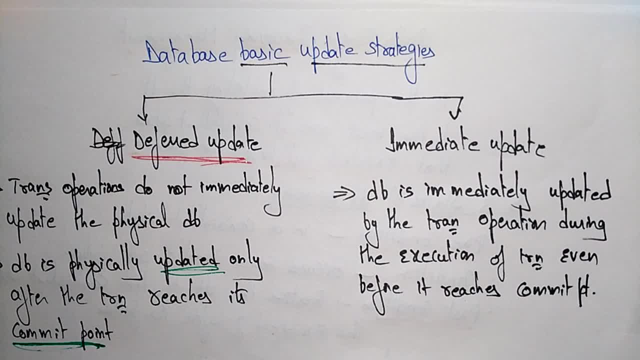 what document you are doing something on word document if you are having the automatically save options in your word document. so whatever the files you are file, you are typing on the word document, it's automatically updated with this like means with the timeline means: after every five minutes, it's automatically updated. 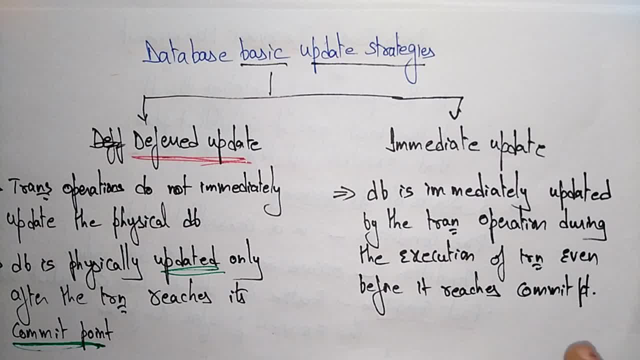 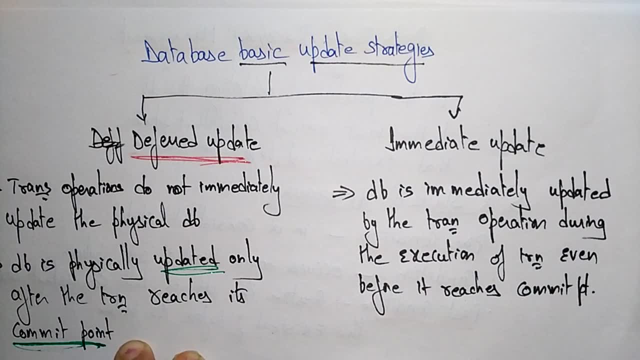 even though you didn't save the file. if you are, that is, the immediate update means whenever you're doing the operations, it automatically updating, so, whereas in deferred update it is not you reach until you save. the button save the file, it won't save the data in your. 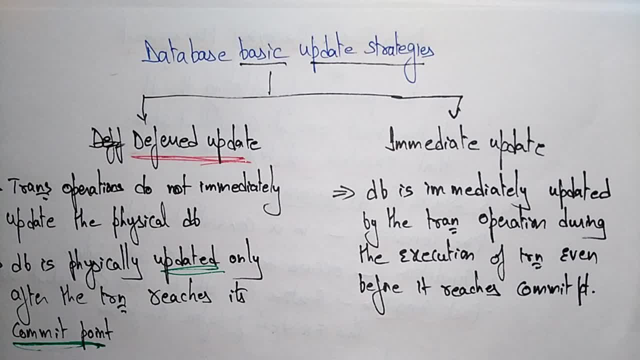 database, just like if you, if your Word document Microsoft Word doesn't have any save option means automatically save whenever you save the file, then only it saves the content. okay, this everything will be after saving. so it automatically saves in immediate update after every five. five minutes, whereas in deferred. 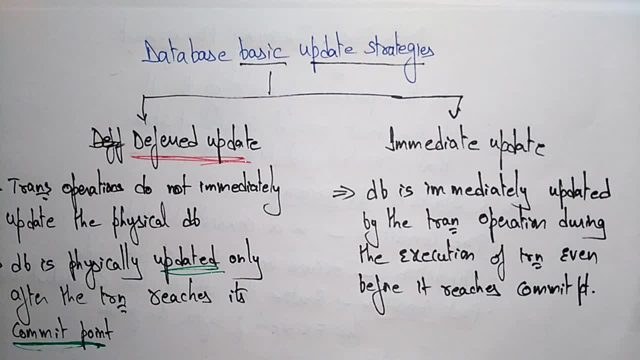 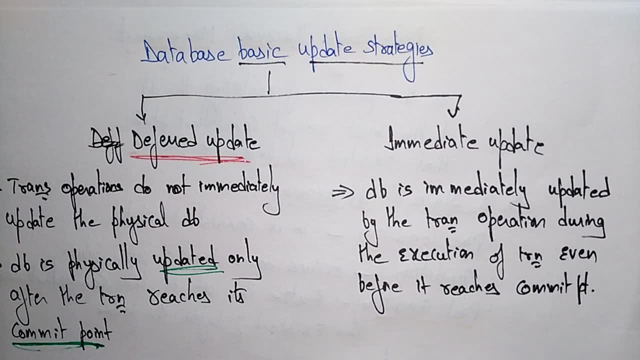 update whenever you save it as it reaches the commit point, then only the database will be updated in immediate while you are doing the operations. the transactions will. before it reaches the commit point, it will be updated. so that is the main difference between the deferred update and immediate update. so 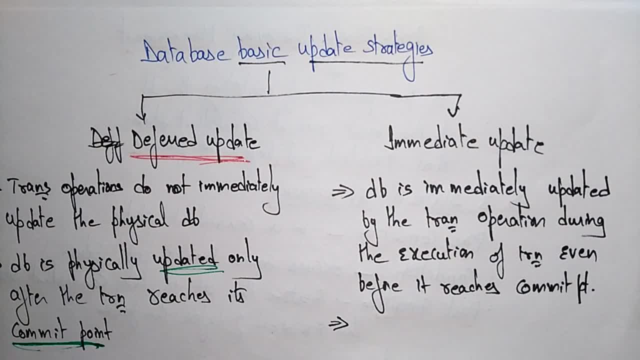 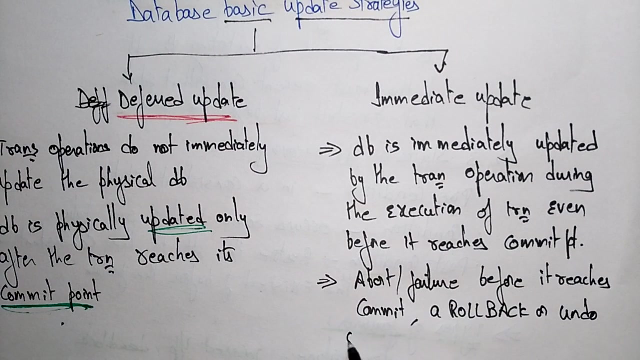 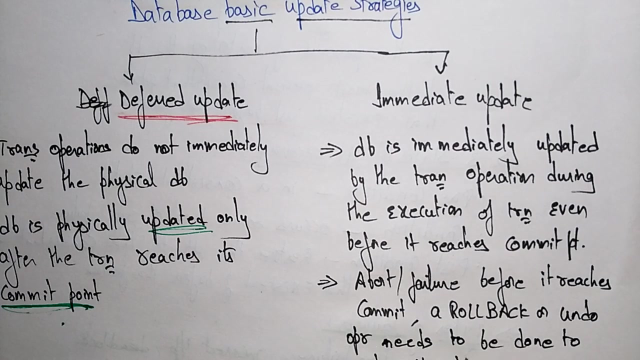 in case of transactions or aborted failure before it reaches commit point. suppose your transaction is abort or failure before you reach the commit point. before it reaches commit, by using a rollback or undo operations or undo operations or undo operations needs to be done to restore the database to its consistent state. so 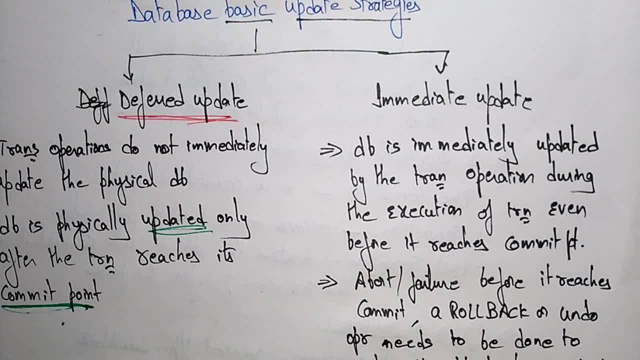 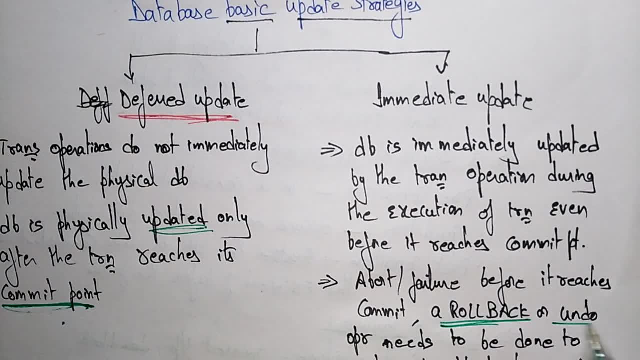 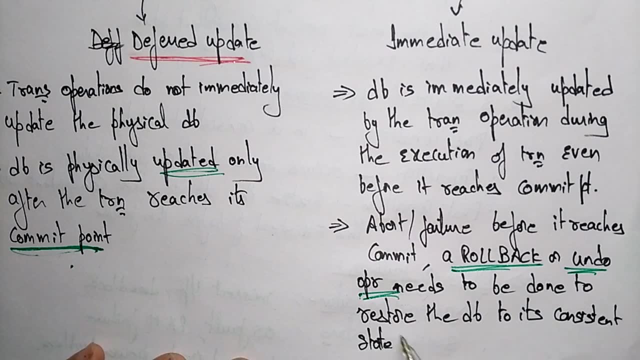 whenever, suppose suddenly your say your system may occur failure, whenever your transaction is aborted. so in that case, if you use just rollback or undo operation, so whatever the data that is in consistent with consistent state before the before failure, that will be restored. ok, the restore the database to its consistent state by using the rollback or